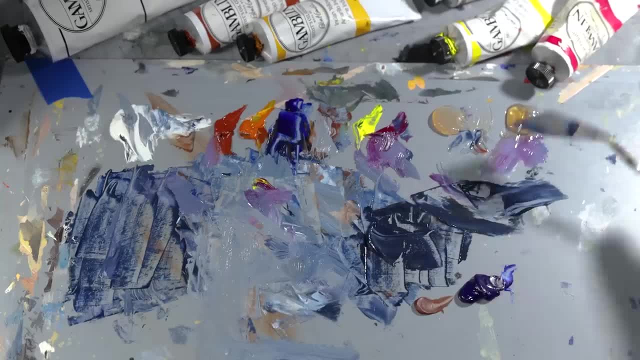 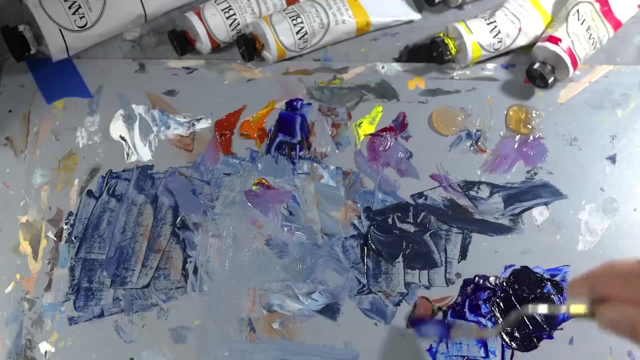 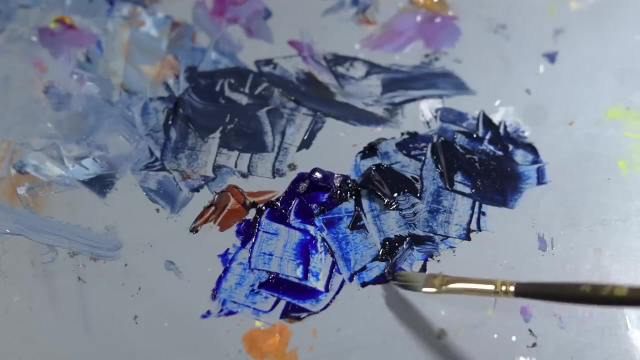 It's called a style stick or a makeup sponge, would honestly work just as well to sort of erase some of those areas where I covered up my drawing. With the background still wet, I mix a dark color and begin filling in some of the shadows and dark portions of the duck. 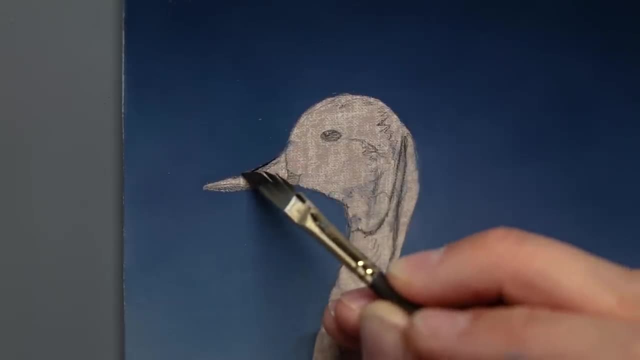 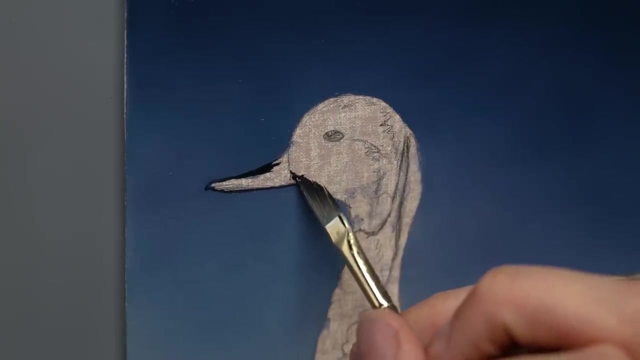 So I started with the bill and then slowly worked my way into the head and down to the body eventually. So this technique of painting- Painting wet and wet to achieve what I feel is a better result as well as a more efficient process- really just comes down to two things. 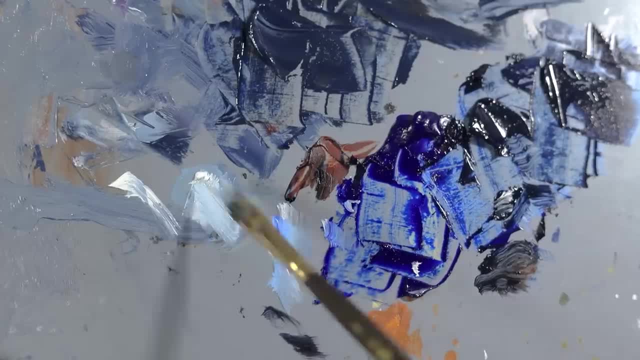 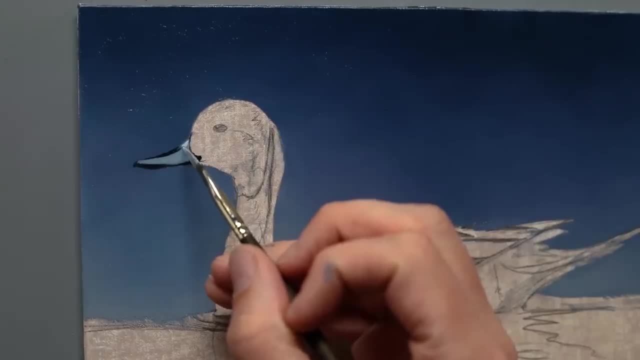 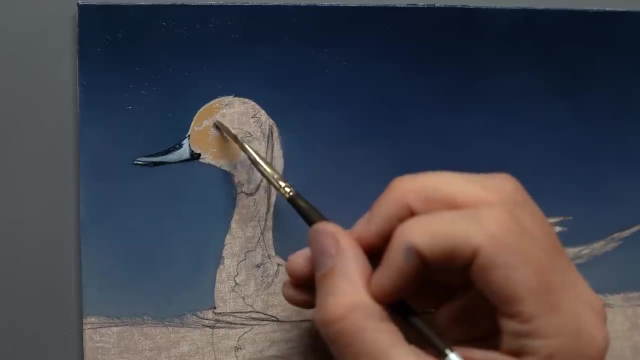 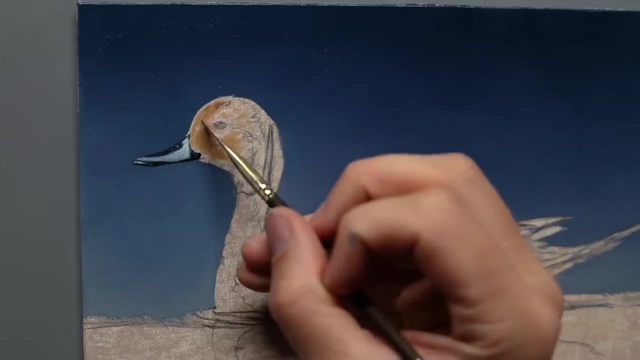 Number one was my mindset and number two was the viscosity of the paint or the consistency of the paint. I think when it came to the mindset that I had about painting, I was sort of putting pre-established limitations on myself and my abilities. I'd always just assumed that I had to layer paint a lot of times- mini layers, in order. 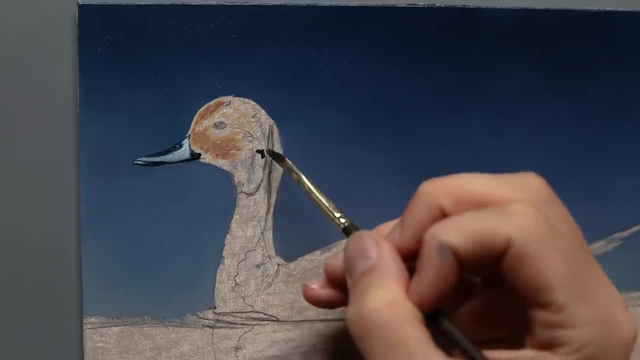 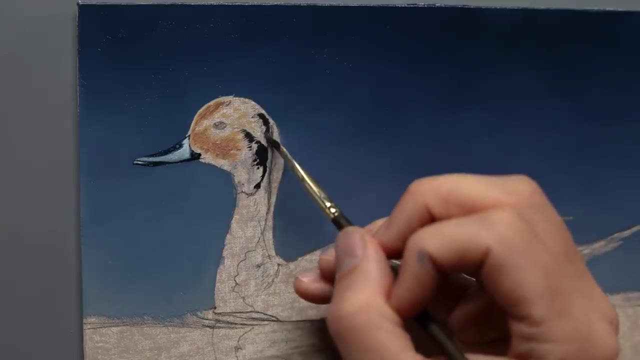 to achieve a certain effect, especially realism, And I never really gave it an honest effort to try and paint everything in one layer or wet and wet paint. I didn't really think that. I didn't think that I didn't think that. 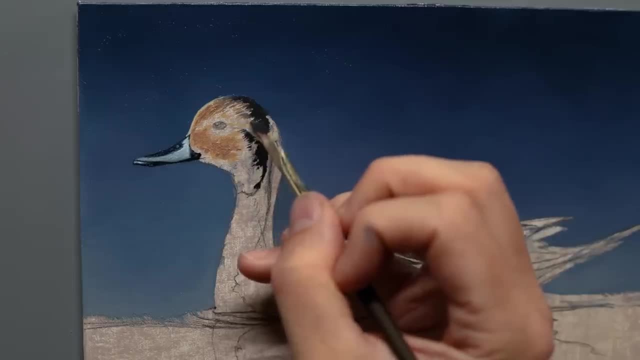 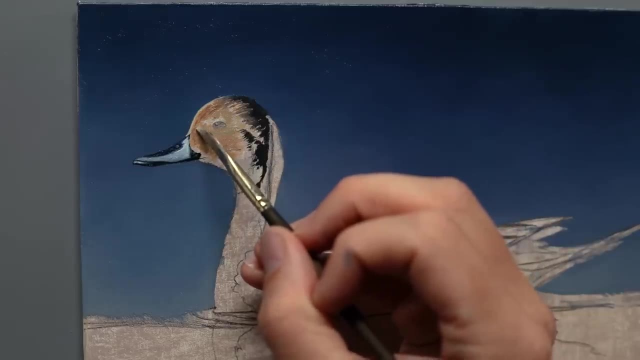 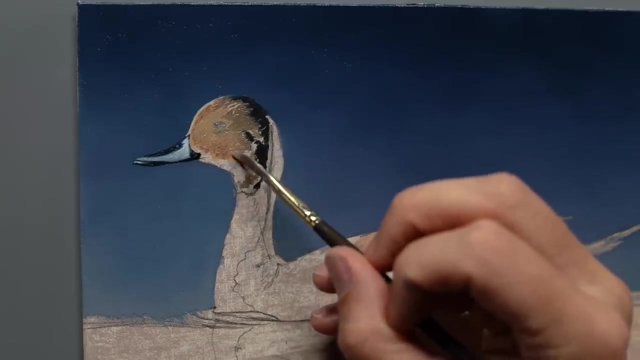 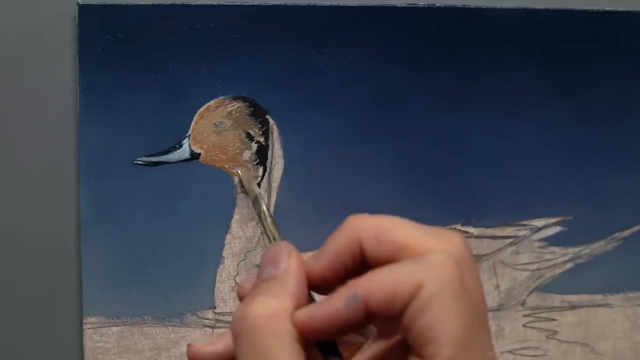 I didn't think that it was quite possible to get something to the point where I was really happy with it without having to use layers. So I feel like I wasn't really giving myself the opportunity to try or the chance to prove myself wrong, And so when I begin this whole process of trying to find a new way to paint this in 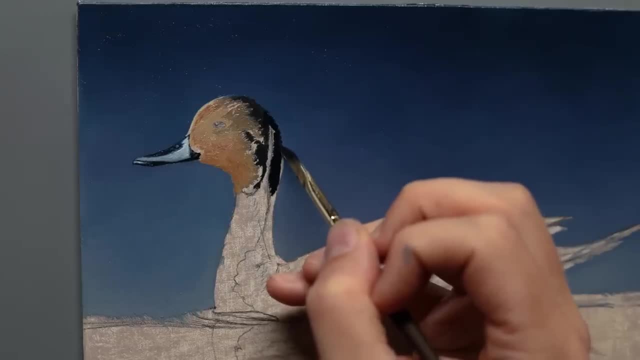 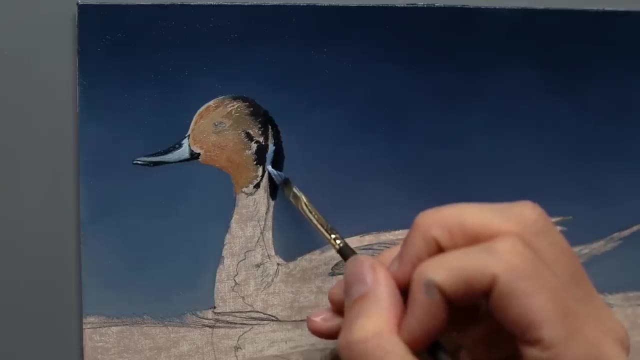 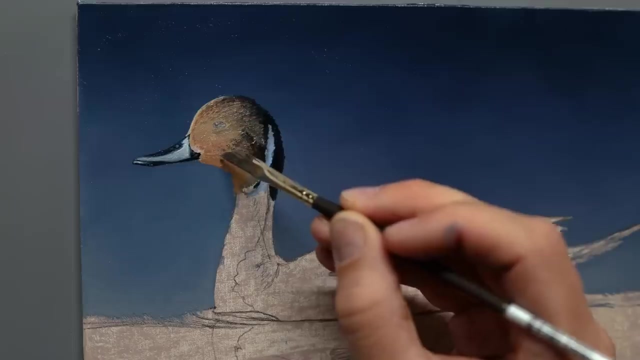 all in one layer. I ran into, of course, a lot of difficulties, And that really forced me to challenge myself and to try new techniques and new, different methods. I experimented a whole lot, And that brings me to the second major thing, which was the consistency of the paint. 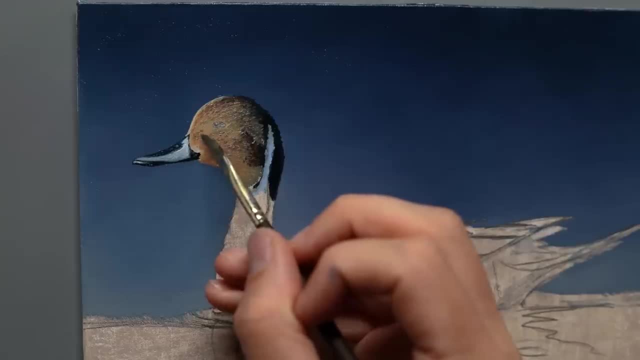 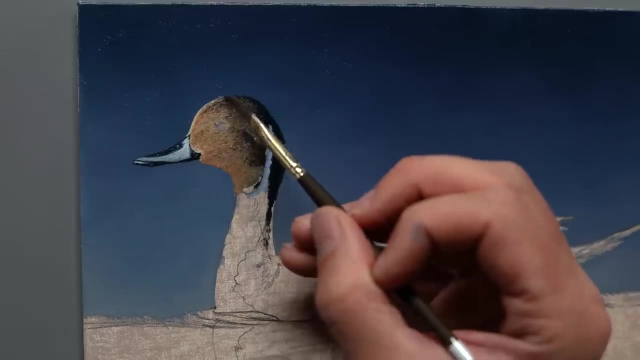 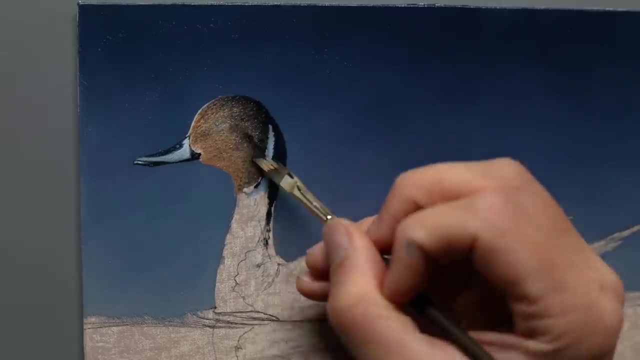 I began to realize that the reason why, when I painted wet and wet, it was not turning out right. It was either muddy or things would just build up in a way that I didn't want them to appear. There's a number of things that can really go wrong when you're trying to mix all these. 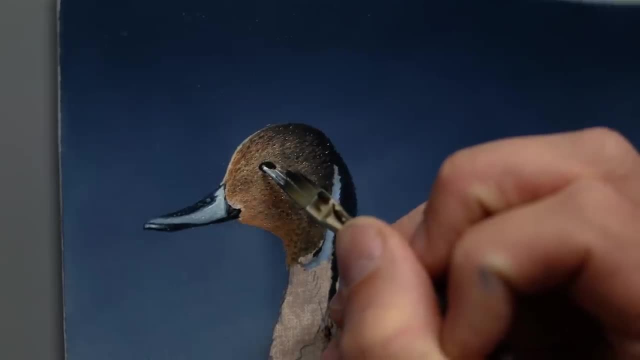 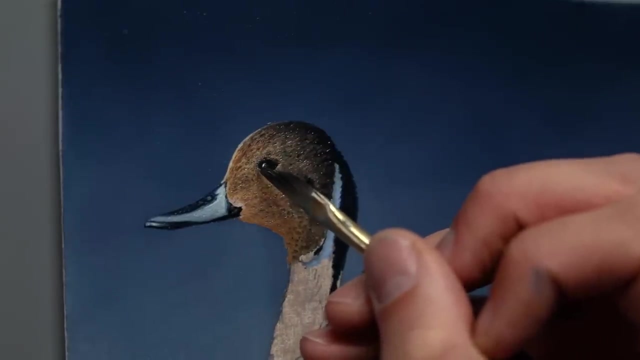 paints together in one. But I begin to discover that if I made the paint a lot thicker and use less medium, that I could layer the paints onto each other rather than have them totally blend into one another. So it allowed me to start to separate colors as I added them to the canvas. 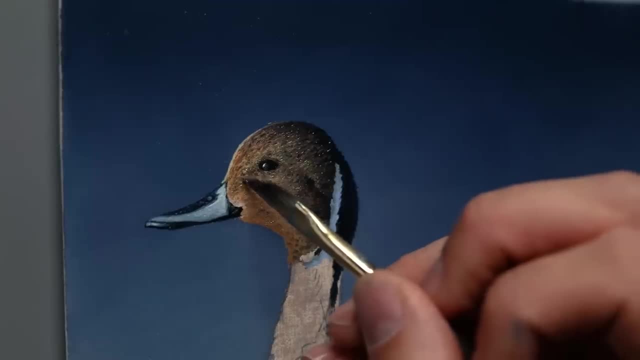 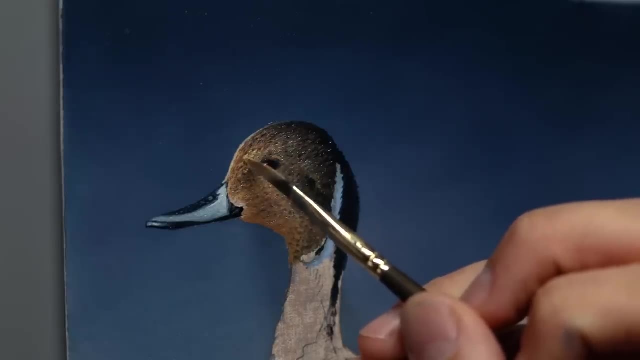 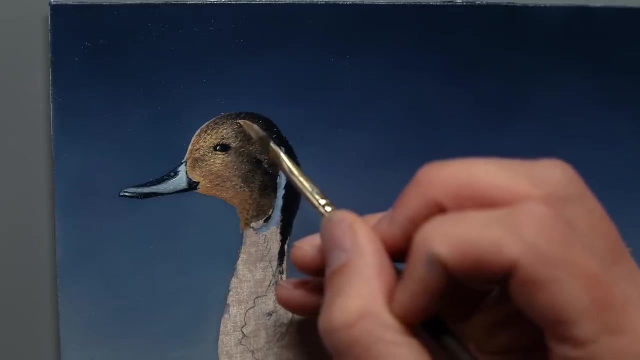 So that got me thinking about trying differently Different types of mediums as well, Mediums that also have a different amount of viscosity to them. So I tried both traditional mediums that I would normally use, like Liquin, and then also mediums that were thicker, like Liquin and Pasto or Gamblin Neomaglip. 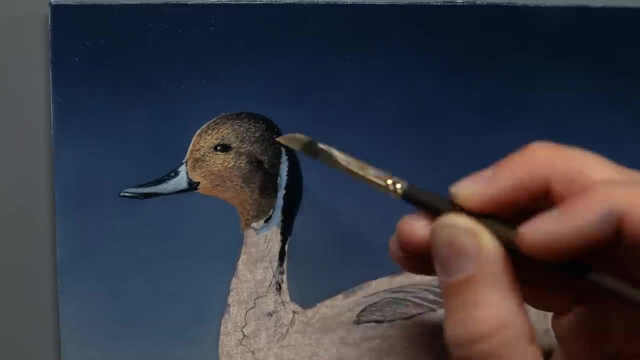 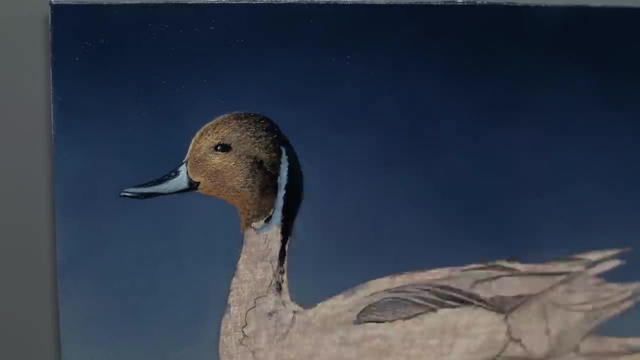 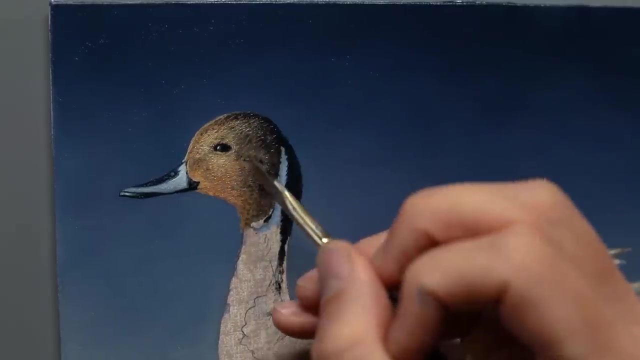 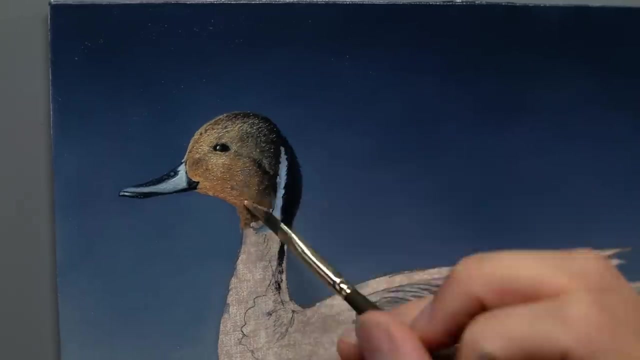 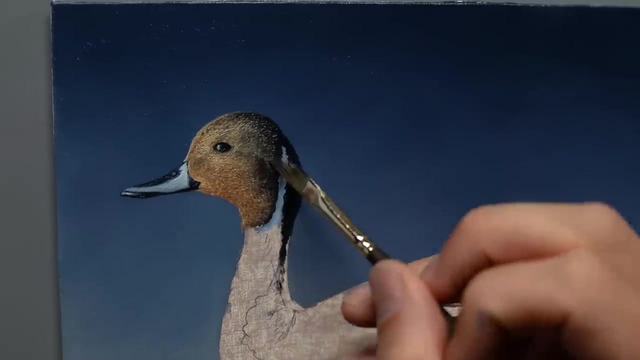 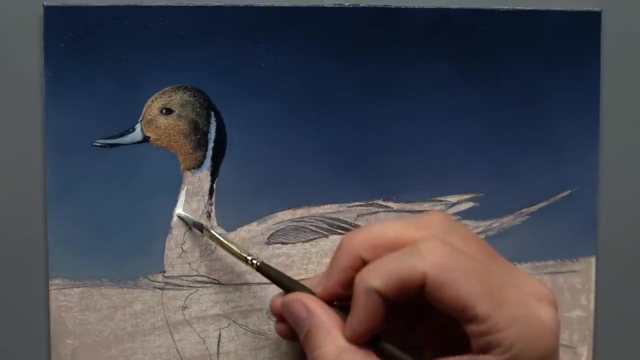 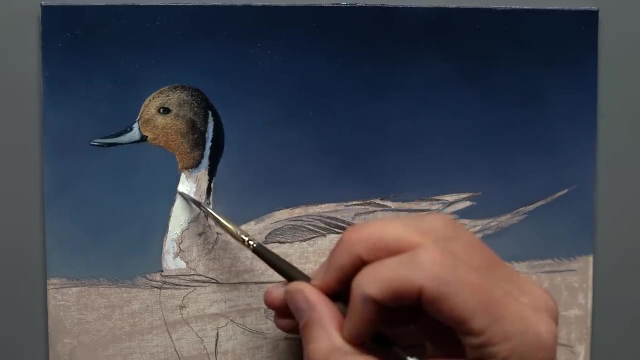 And that began the process of me discovering that there were different ways to do this. To sum it up in short, I basically just use very little medium and apply a thicker roll of paint. Then I add a little medium to the canvas first, And if I'm painting something super detailed like the chest, the side of this duck, where 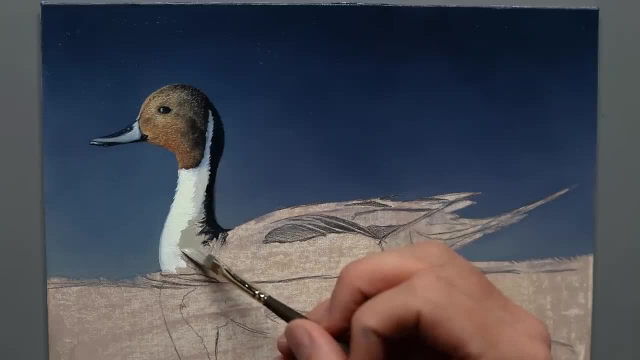 there's all kinds of striping and patterning going on. I'll start with the most common color in the body, So a light gray with a touch of warmth to it, And that's a thick, wet layer of paint that. then I add a little medium to some of the 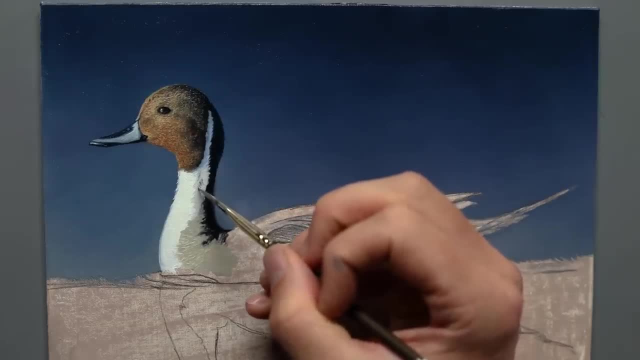 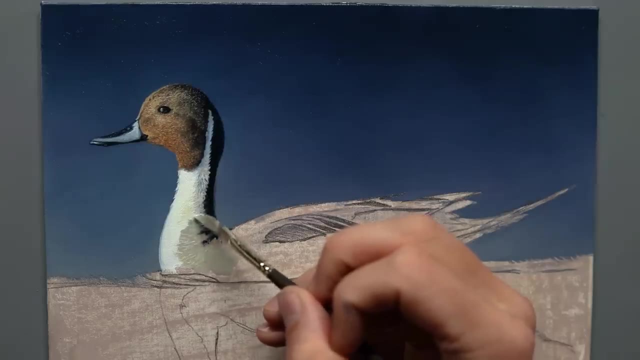 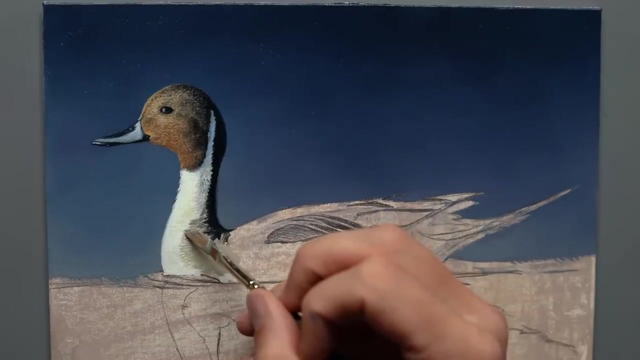 dark stripes and some of the light stripes go back over the top and that thick paint underneath And then I actually blend as much as if I used a lot of Liquin to begin with in that first initial base coat. I also found that Liquin and Pasto can really help you layer wet paint over wet paint as 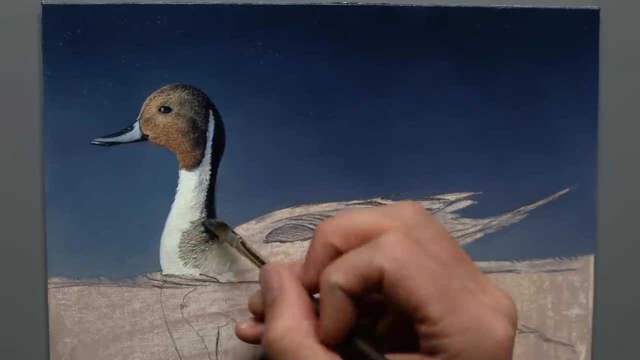 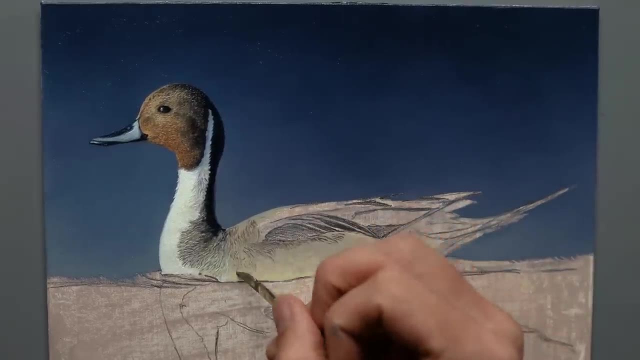 well, because of the fact that it's a thicker medium, It just doesn't want to fluidly blend in anything that you're applying it to. So what I do is try to use Liquin Original a very small amount to see if that will give. 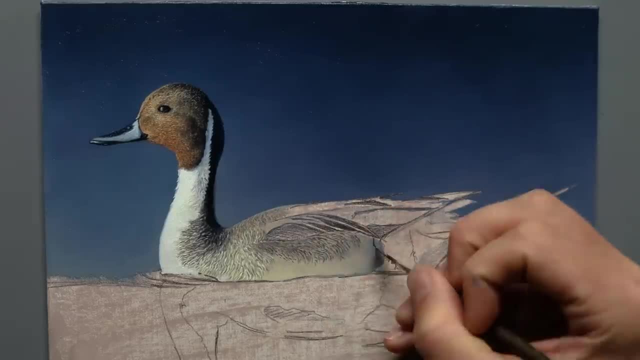 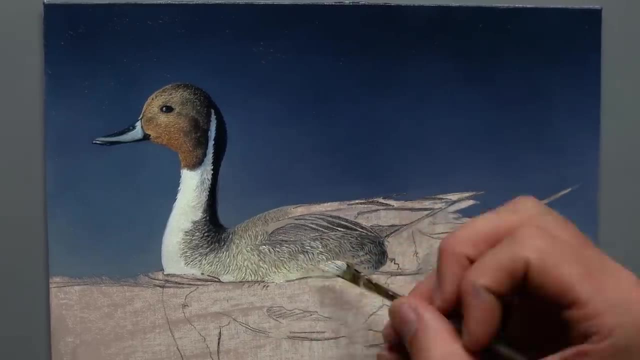 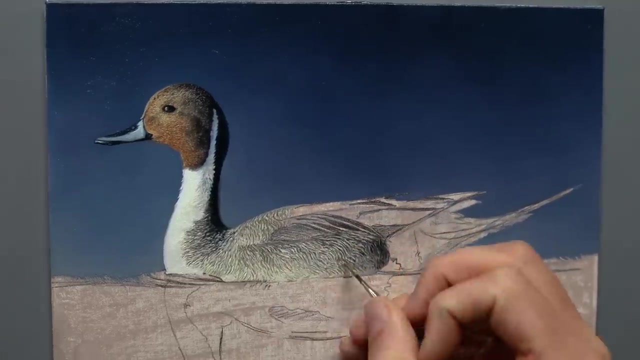 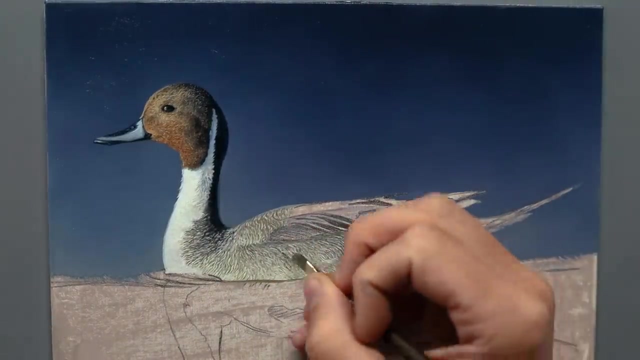 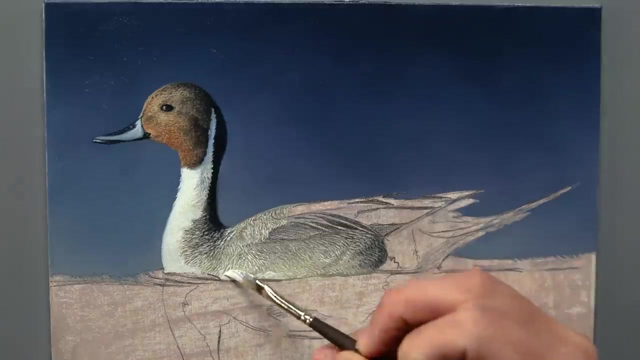 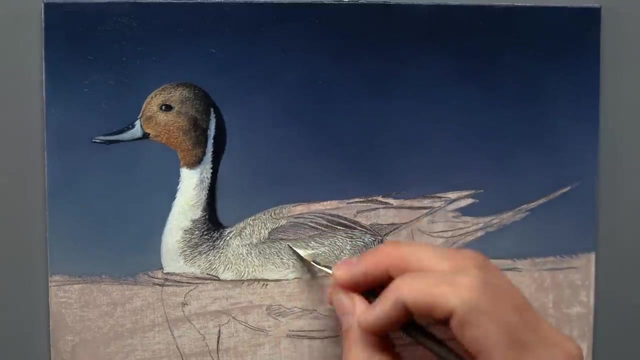 me the ability to paint over the top of wet paint And if that doesn't work I'll add a little bit of Liquin and Pasto and that can really help me achieve those effects. But all of that with the mediums and the consistency of paint doesn't really solve. 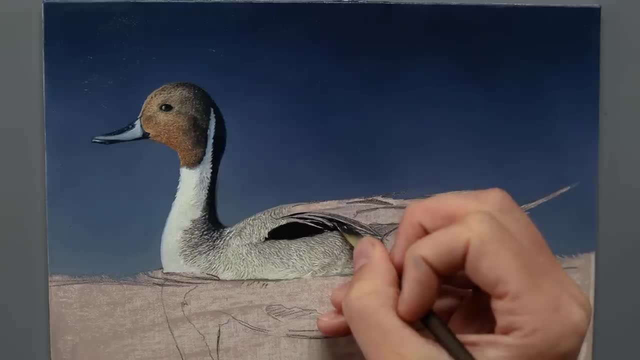 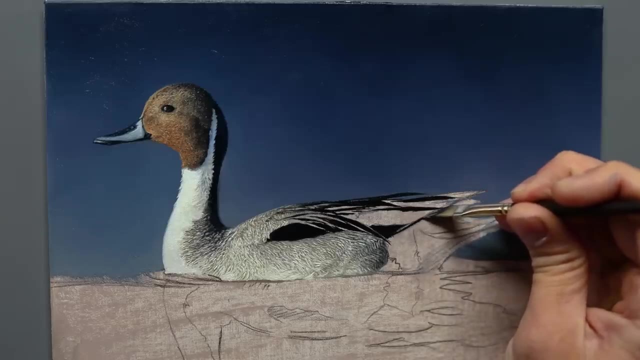 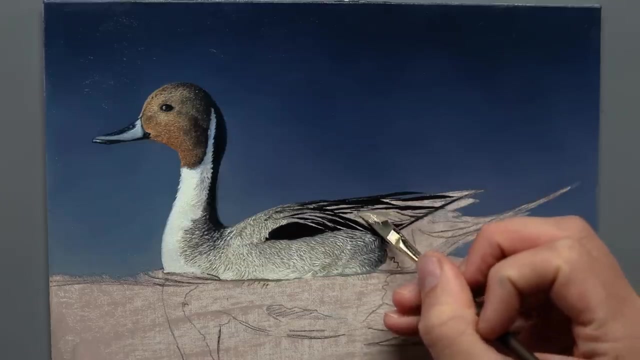 it all for you. It still circles back to the mentality that I had before versus now, And that literally was just telling myself that I'm going to sit down and finish this the way that I want to And I'm not going to stop working the paint until I'm satisfied. 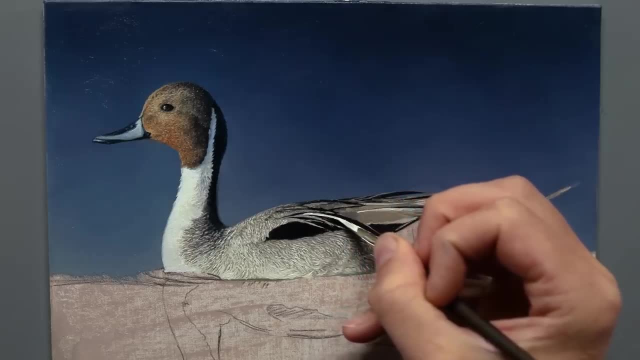 And as long as I have a good, accurate drawing on the canvas sort of laid out for me to where I know where everything is supposed to be, I found that if I had the discipline to see it through that I was capable of doing it. 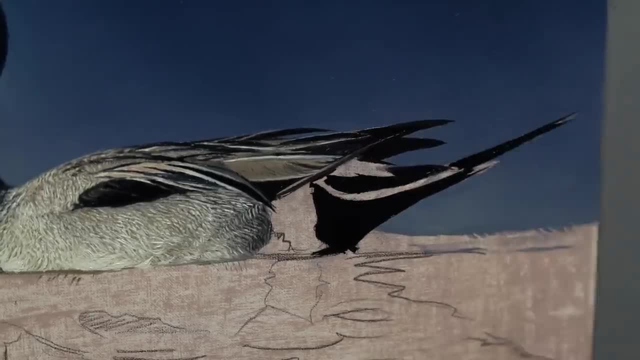 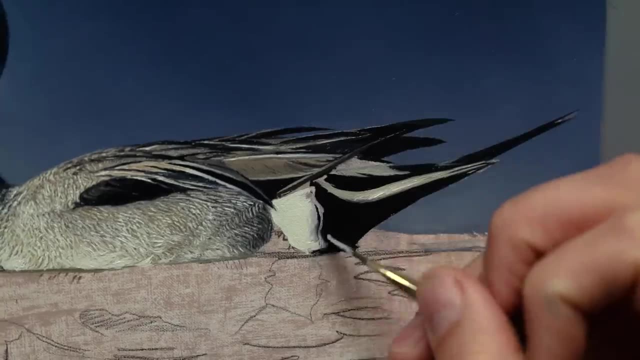 So, in short, I think what I'm trying to say is I just got a lot more discipline and I just made up in my mind that I was going to work a lot harder. I was going to work a lot harder to achieve the effects I was after while working wet. 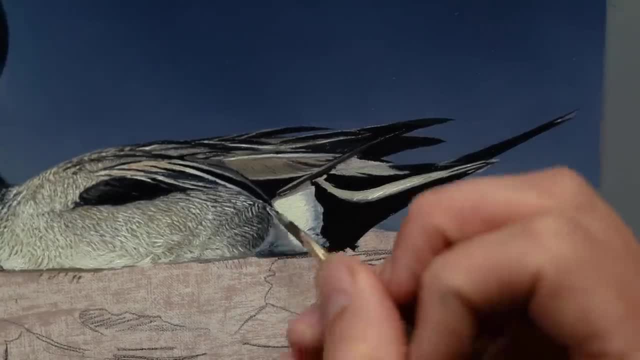 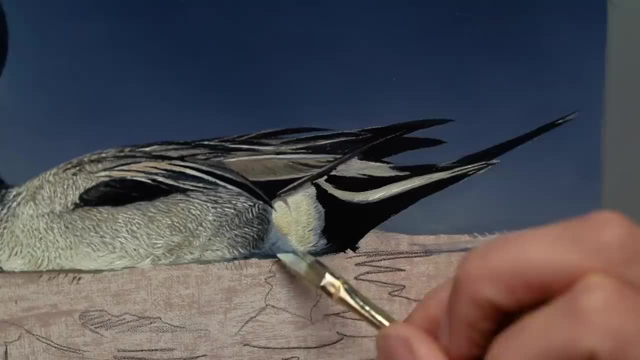 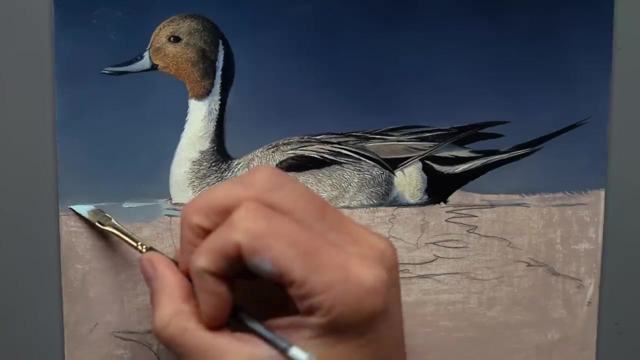 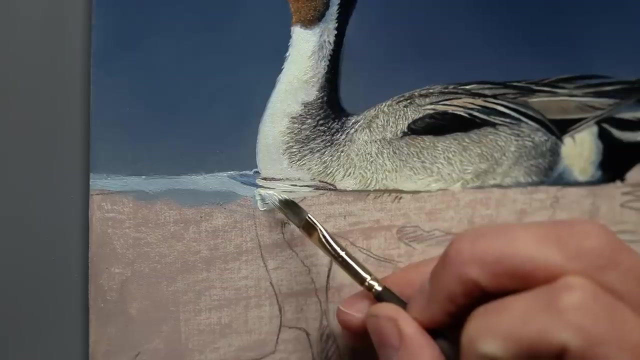 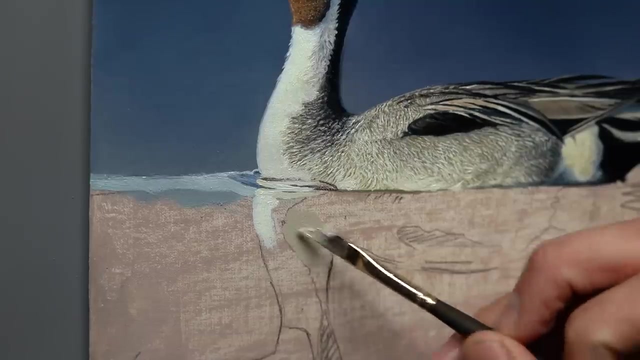 and wet. This process that I've developed for myself seems like it's taken eternity to finish. It's taken forever, It's taken years to figure out, And I know that it might not be helpful for all, but I think it's a good reminder to keep. 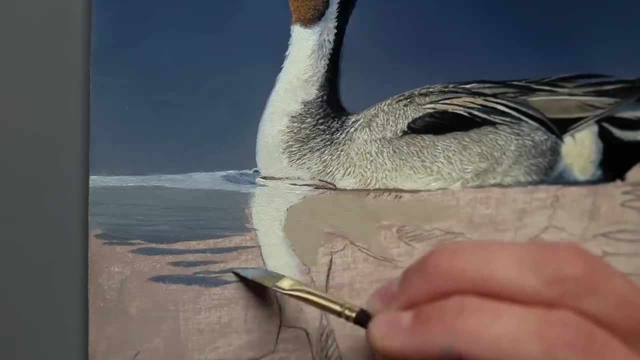 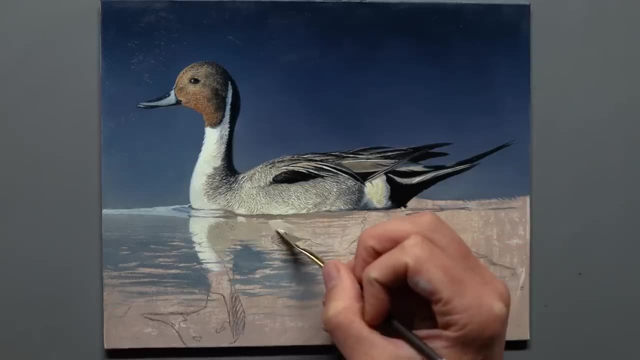 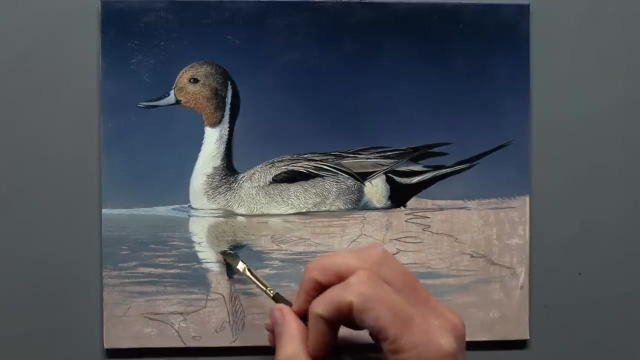 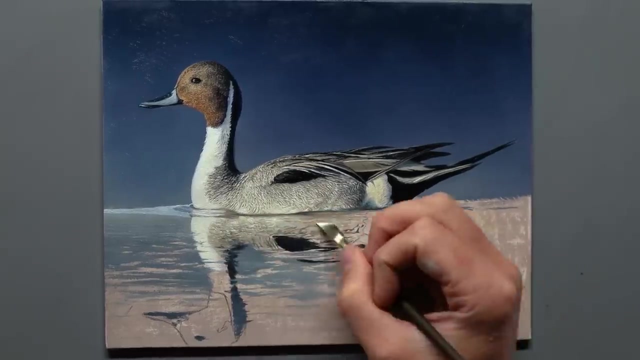 striving to try new methods and new techniques. Keep striving to challenge yourself and be willing to push through the constant frustration of painting- And, believe me, I've been frustrated more often than not. There's very few joyous moments When I'm actually manipulating the paint on canvas. it's usually quite stressful.